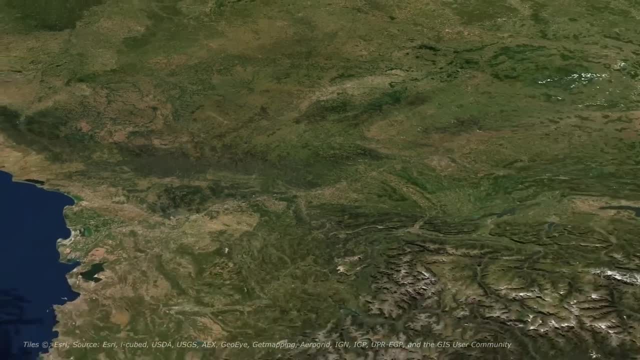 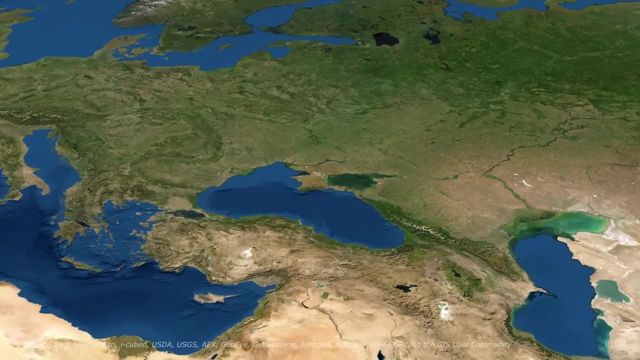 This video was brought to you by Morning Brew. The reason we define Europe as its own continent and not some sort of giant peninsula in Western Asia is because… history- Perhaps it is appropriate- I talk about these islands right here in the Aegean Sea. 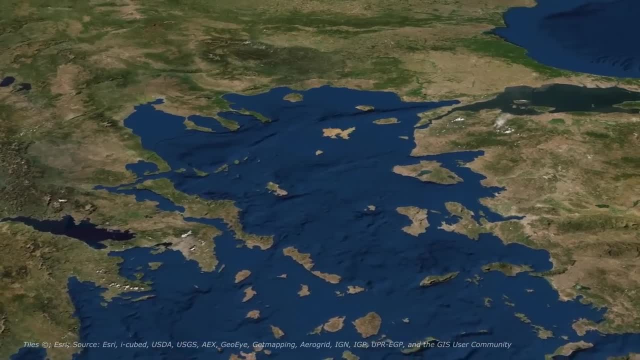 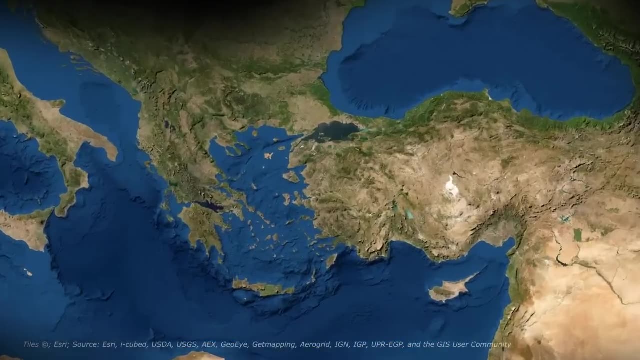 as it was ancient Greek cartographers who first made this distinction In the 6th century BC, when all the lands people in this general area knew about looked like this. there was this one guy from Miletus named Anaximander, According to several Greek, 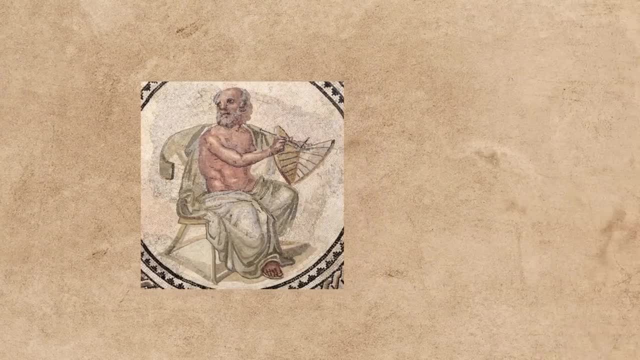 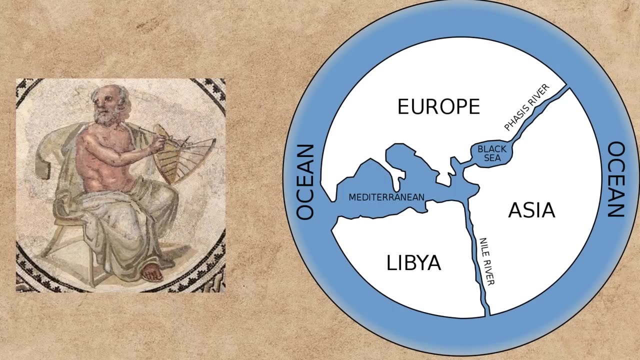 cartographers and philosophers that came after him. Anaximander was the first to ever publish a true map of the world, and this world map had one huge distinction, well, I mean, aside from being existent when all others at the time weren't. 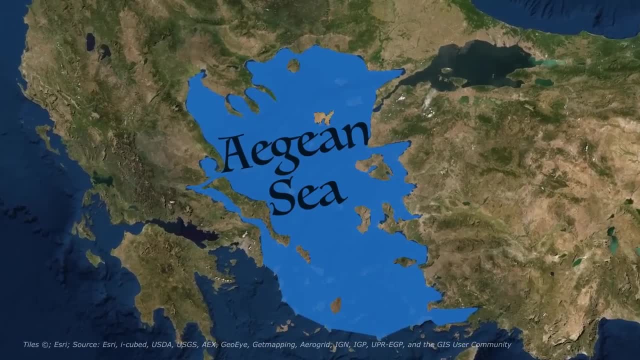 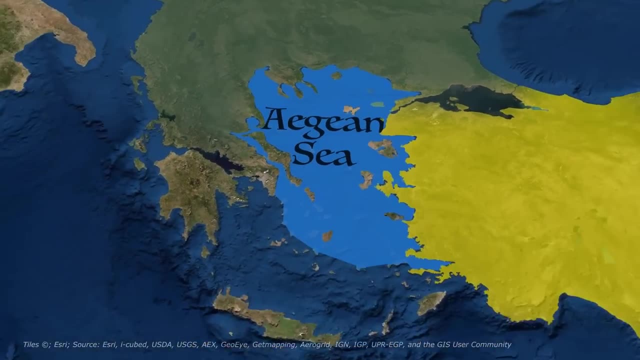 To the ancient Greeks, the center of the world was the Aegean Sea and its hundreds of islands. anywhere to the east of the sea was Asia, anywhere to the west was Europe and anywhere to the south was Libya. This concept gave a lot of people a lot of different ideas on. 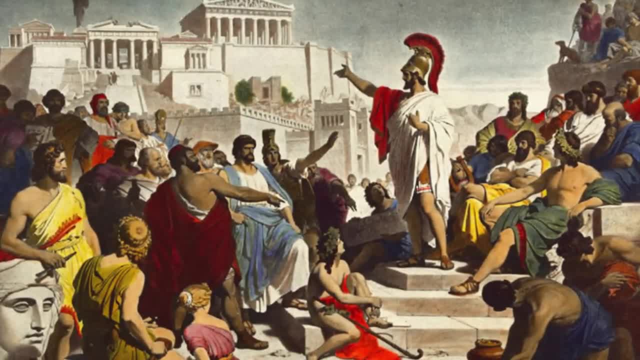 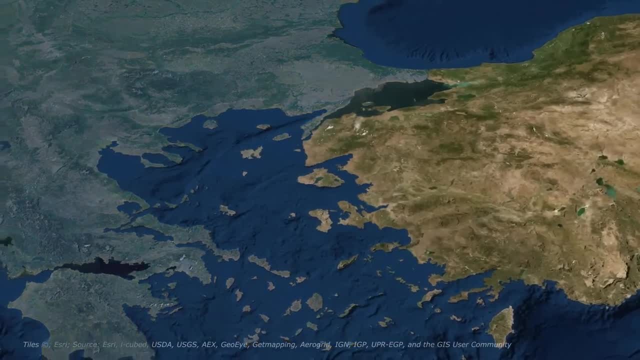 what role the Greeks themselves played amongst the different continents. While some historians argue that perhaps European Greeks used it against those who had fallen to Persian domination, others at the time excluded the Aegean islands and the Peloponnese, and therefore the Hellenic. 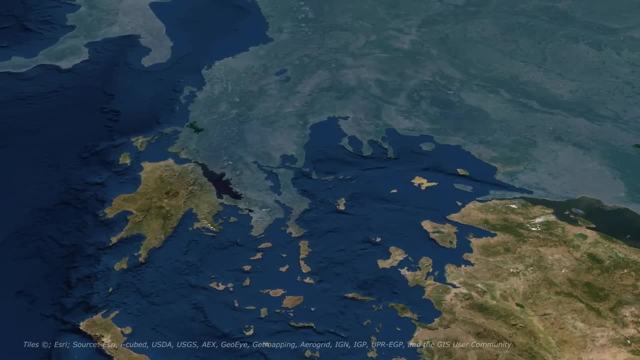 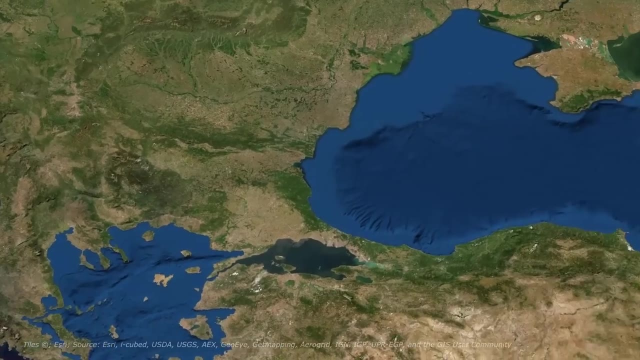 peoples themselves from this continental model altogether, with the concept of Europe being more connected with the non-Greek Thracians to the north. But even back in this time, people knew that Europe and Asia were in fact connected by land north of the Black Sea and had already 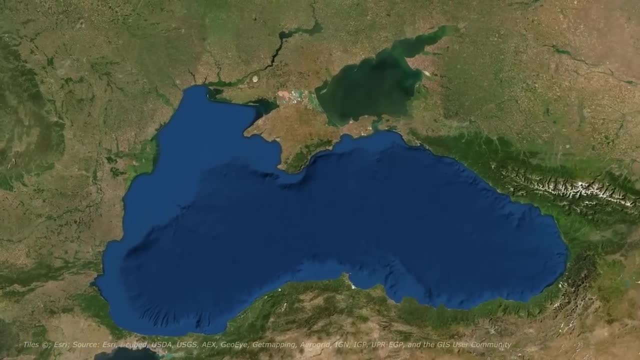 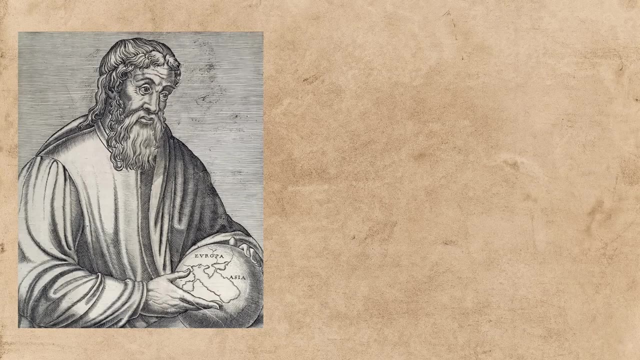 begun to question why two conjoined regions would be their own separate continents. Talk about the original Euroskeptics Writing in the first century BC. Strabo made the observation: in giving names to the three continents, the Greeks did not take into consideration the 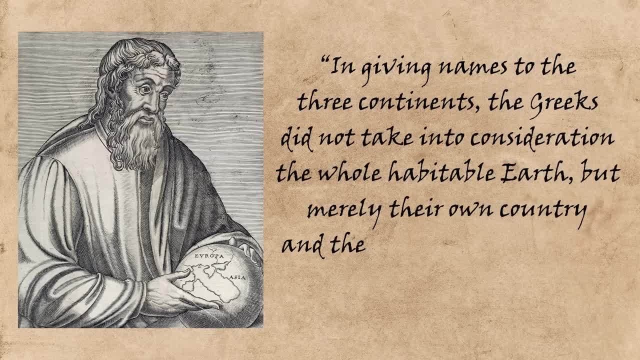 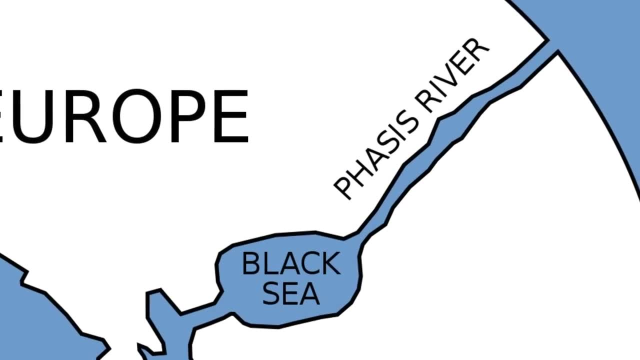 whole habitable earth, but merely their own country and the land exactly opposite, And I'm not going to go into too much detail on this, but if you're interested, you can go ahead and check out the video description. Anaximander defined the border between Europe and Asia as following the Fascius river. 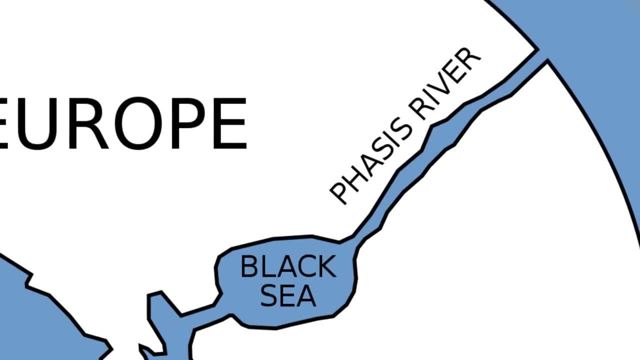 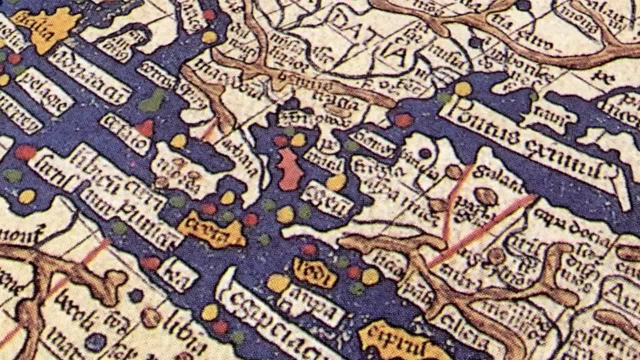 and Georgia until it reached the Caspian Sea… uh, somewhere, and the border between Asia and Africa as the Nile. Throughout the Roman era and the Middle Ages, European cartographers largely followed Ptolemy's version through the Turkish Straits into the Black Sea, then through the 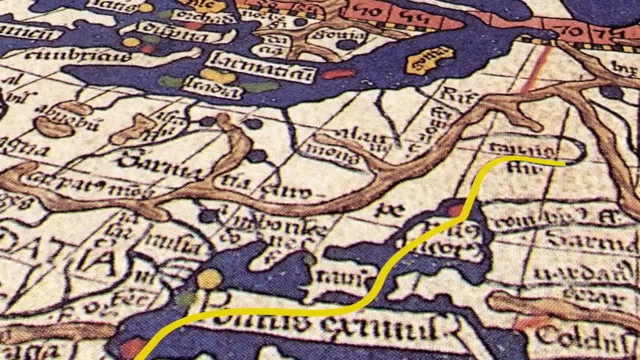 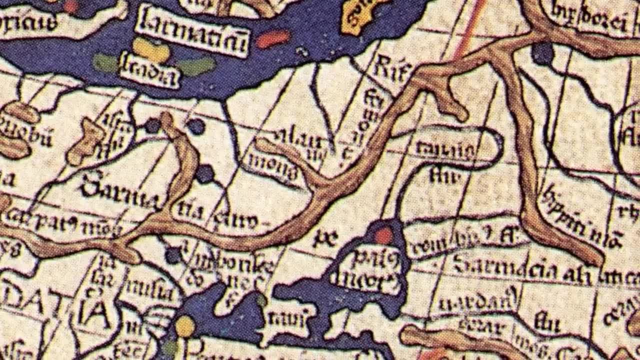 Kerch Strait into the Sea of Azov, and then following the Don River to… wherever it ended up. However, by the 16th through 18th centuries, this definition was starting to get a bit problematic, as Russia was expanding into. 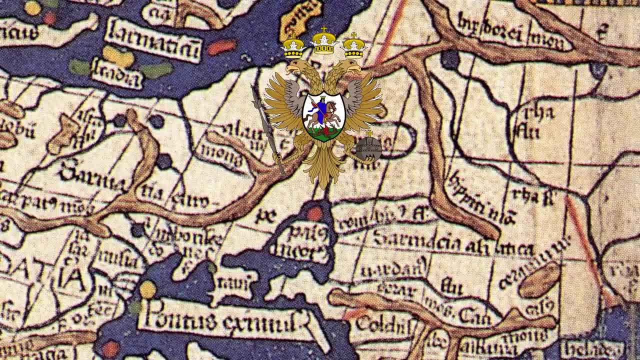 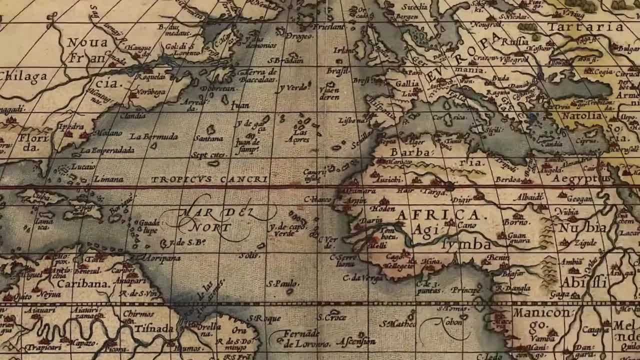 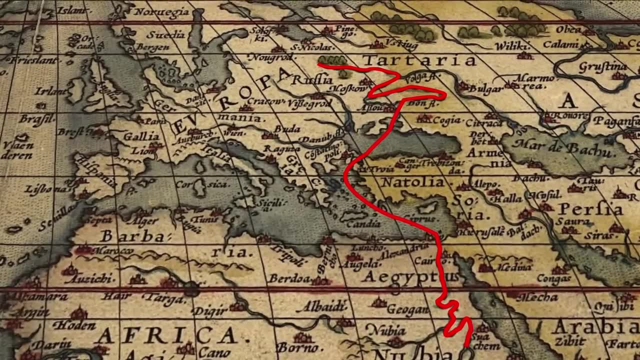 the very lands that the smart dead people in Greece never knew about. As European cartographers came to know about more of the world, including get this, a fourth continent, it became obvious that the Nile and the Don might not have been the best geographic features to separate Asia from Africa and Europe, and thus new dividing lines. 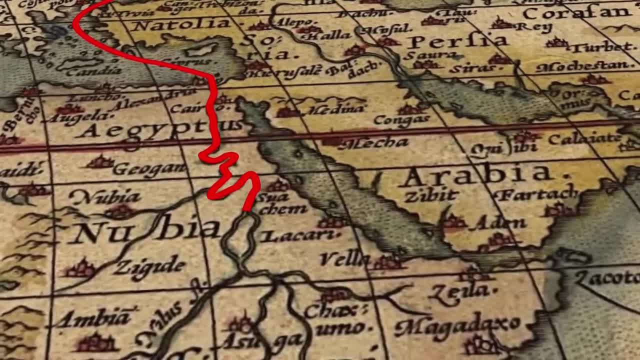 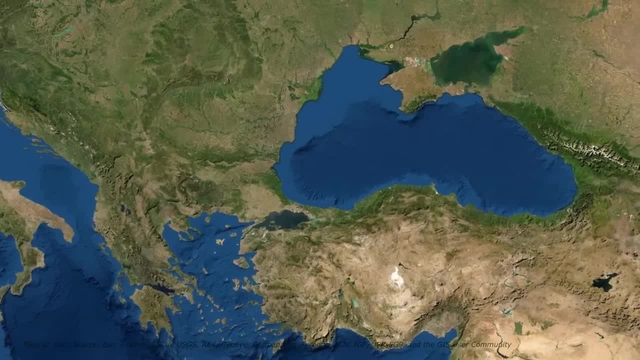 had to be figured out With Asia and Africa. it was pretty easy. You see that huge sea that almost looks like the Mediterranean here. Yeah, put the border there dummy. In 1725, German-Swedish geographer Philipp Johann von Stralenberg, who was also dead. redefined the border to follow the Volga River from the Caspian Sea until where it bends near the city of Samara, also known as the Samara Bend. It then followed the division between the drainage basins of the Volga and Ural Rivers, known as Alpsjussert, before following the Ural. 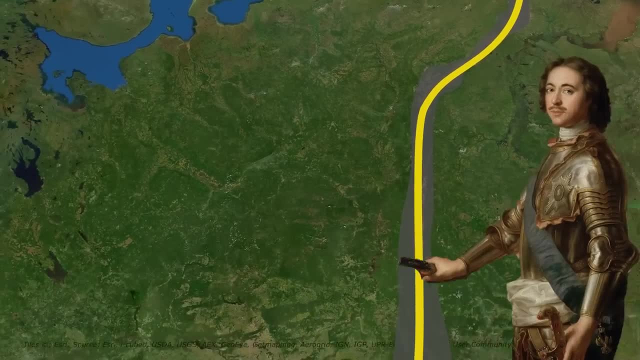 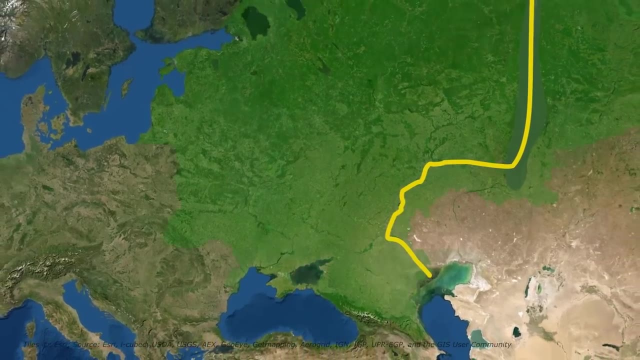 Mountains into the Arctic Ocean, As the Russian Tsar Peter the Great was on his whole. Russia is a Western shtick. Russian intellectuals associated with him basically went sweet. this puts so much more of our country in Europe. look, we're totally Western. check out our new tricolour flag. 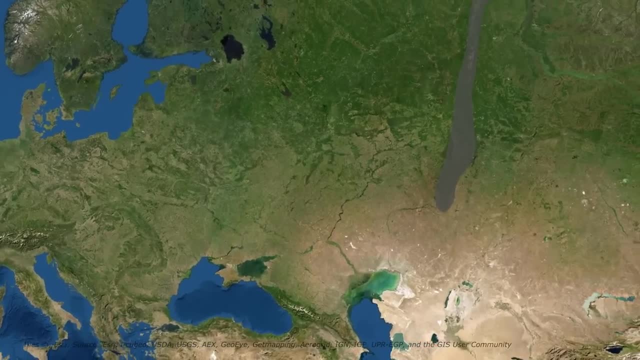 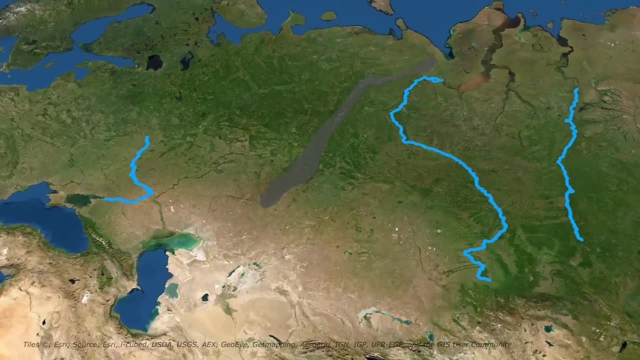 However, other scholars across Russia and the rest of Europe would fiercely debate this idea, with some still wanting to use the Don and others wanting to go as far east as the Ob or the Yenisei. but eventually the Urals were the one thing just about everyone could agree on. 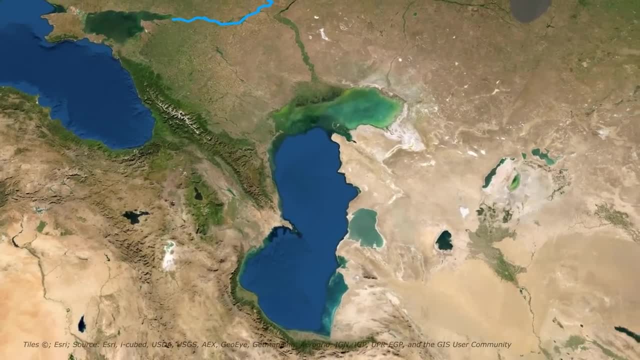 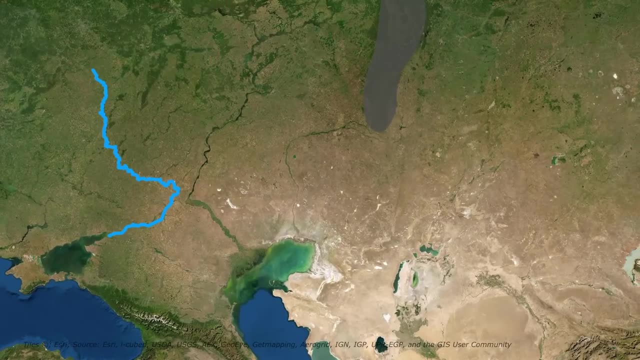 and, to a lesser extent, the Caspian. However, as the universe inherently doesn't care about the whims of some hairless apes who argue over which way toilet paper should be hung, the Urals don't actually extend all the way to the Caspian. Increasingly, cartographers started to put. 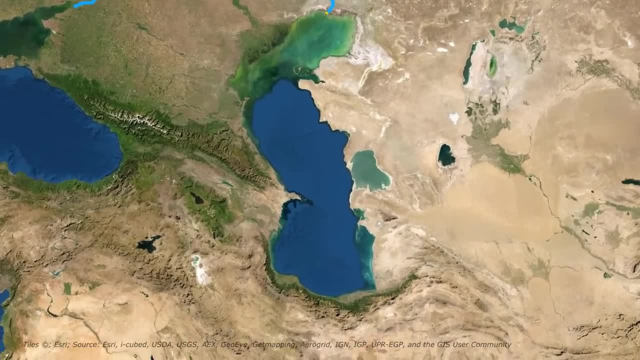 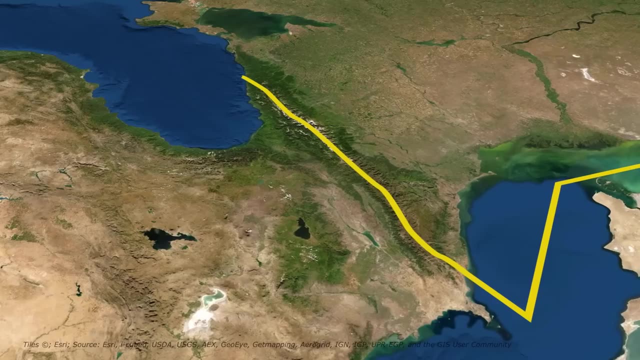 the boundary along the Ural River until it reached the Caspian, going down the sea about two-thirds of the way before turning to the northwest and then going along the Caucasus Mountains instead of any river. But even then the division wasn't completely set in stone with Soviet geographers. 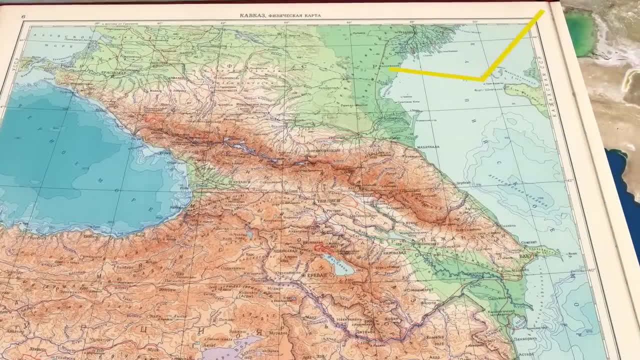 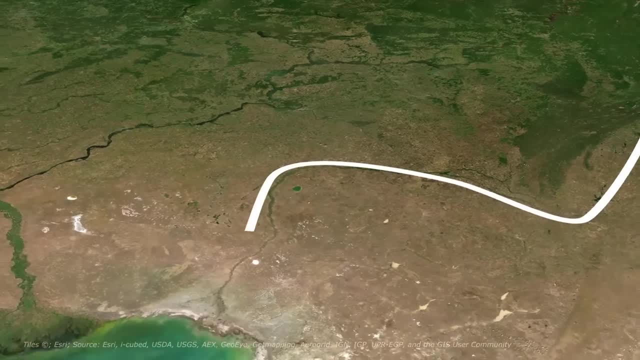 in the 1950s, proposing the divide instead follow the Kumamonish Depression in the Caucasus. Nowadays, the dividing line follows the eastern foothills of the Urals, then the Ural River into the Caspian and then along the watershed of the Caucasus Mountains. 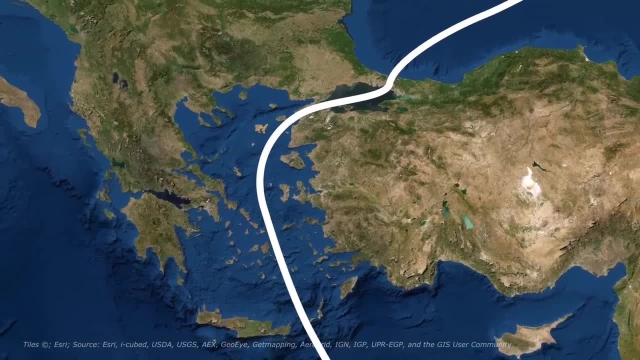 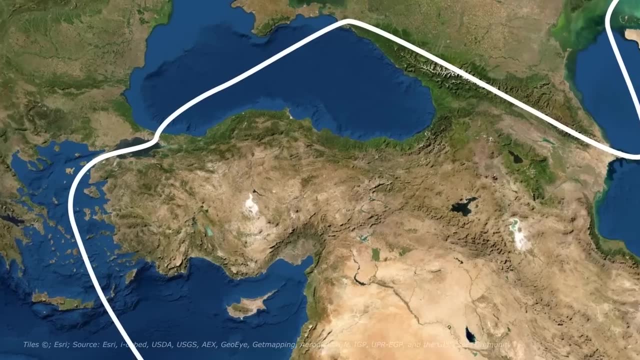 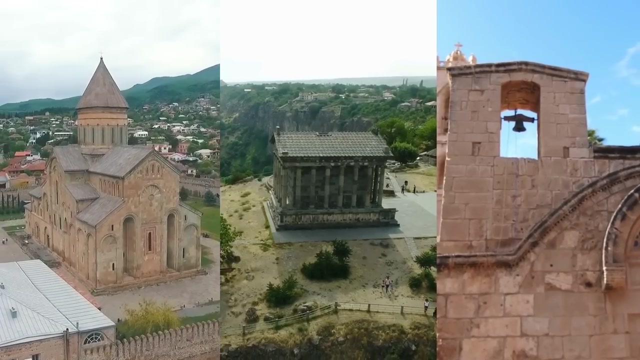 before emptying into the Black Sea and passing through the Turkish Straits, therefore making both Turkey and Greece transcontinental countries. But if this division is all about culture, what about Georgia, Armenia and Cyprus? Culturally, historically and geopolitically, these nations have all had much more to do with Europe. 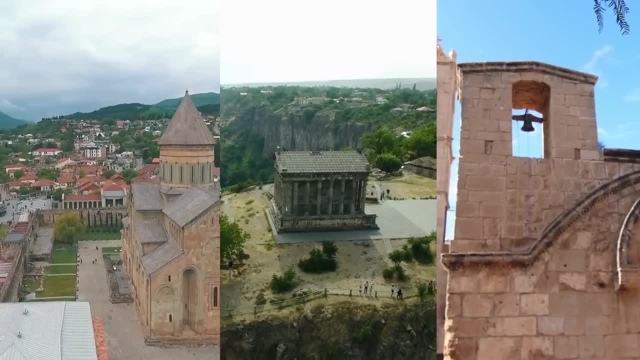 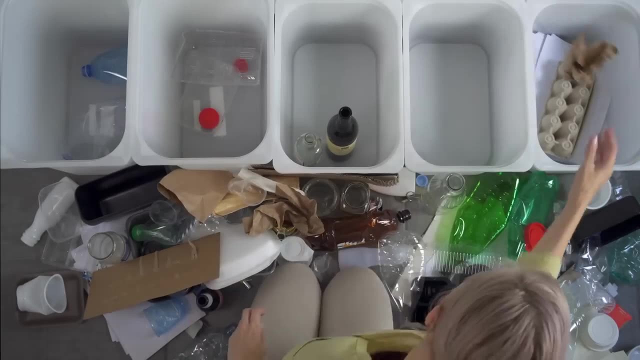 and yet they all find themselves mostly in the middle of the Caucasus Mountains. What I think this sort of tells us about humanity is how even human things evade the human desire to sort everything into neat little categories. The most empirical way to divide a continent, at least without including islands- 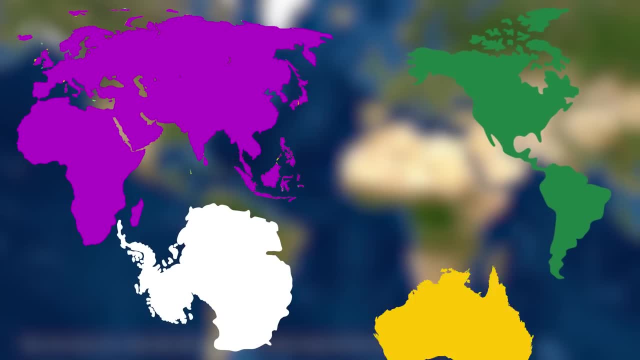 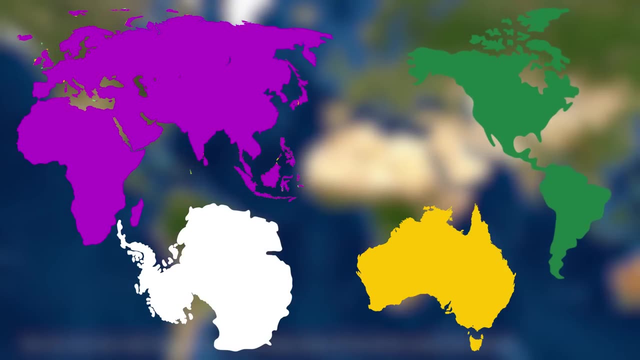 might be to just count Afro-Eurasia, the Americas, Antarctica and Australia, but if we think about it, that's not what most of us use continents for, The way we actually use continents as a way to categorize the peoples and cultures of this mudball. 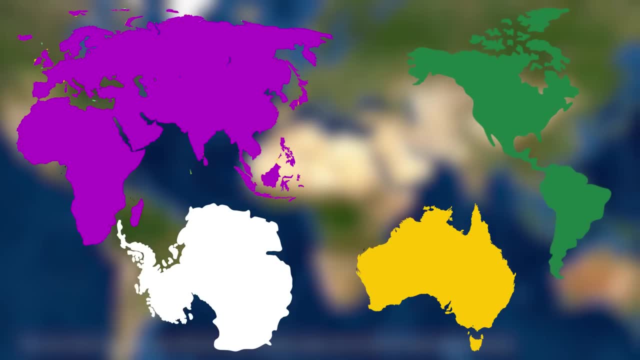 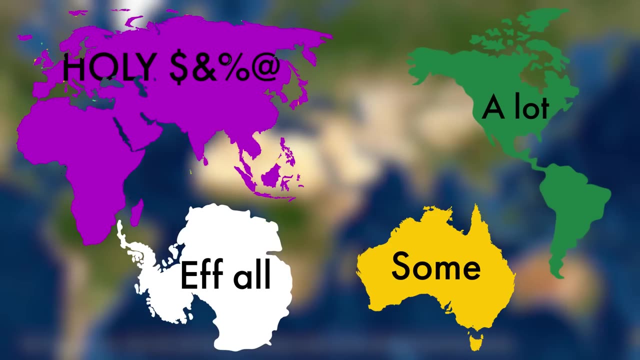 doesn't really jive well with this definition if we only count landmasses with populations of a few hundred, 25 million, 1 billion and 6.7 billion. God, imagine what it'd be like if Europe and Asia had random little enclaves and exclaves within each other. 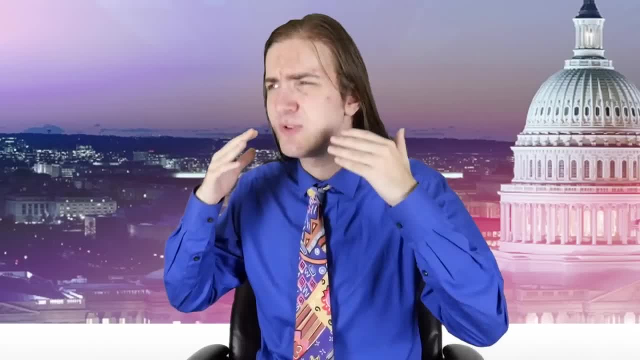 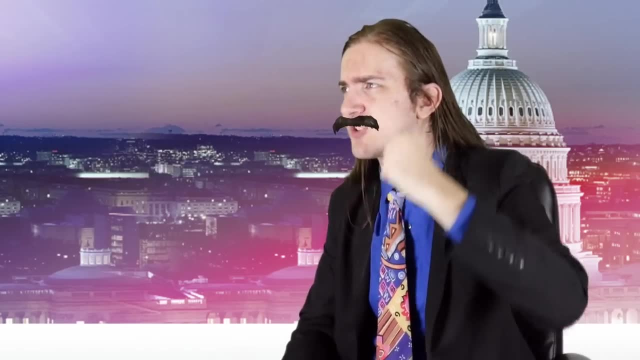 Okay, but you can't just write off the Mariner Valley like that. Um, have you seen what's going on in Arcadia? It's a war zone over there. I don't care about what's happening on Luna or Mars. I want incriminating pictures of Spiderman. 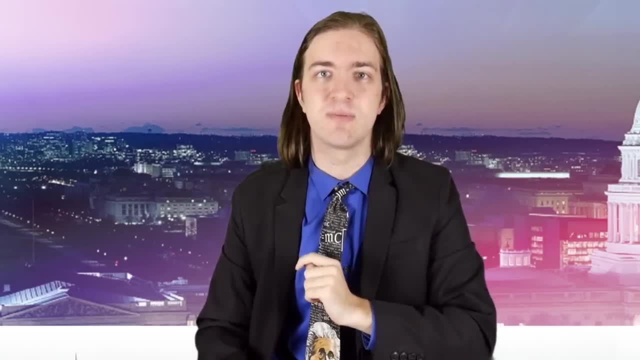 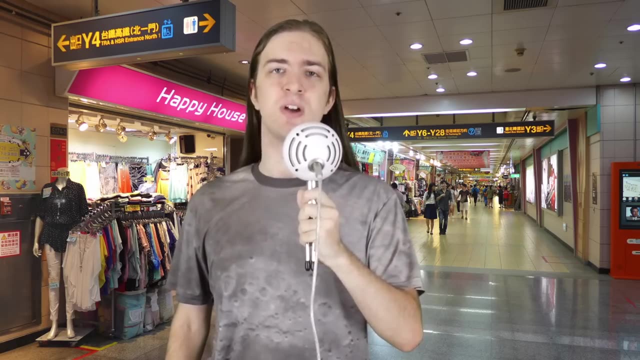 Okay, well, let's tune into our reporter on the scene in Shackleton right now. Thanks, Daryl. the situation in the crater region is actually completely, totally normal, but we still have another 23 hours and 59 minutes left of program to fill. 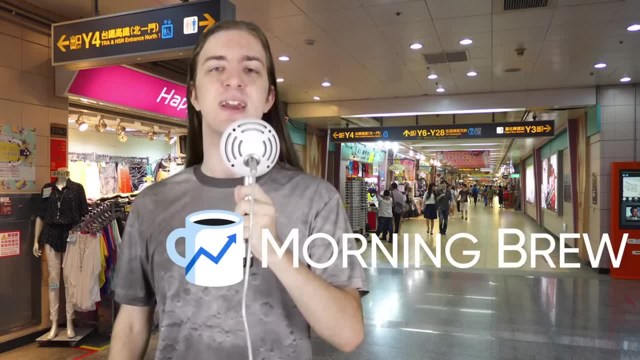 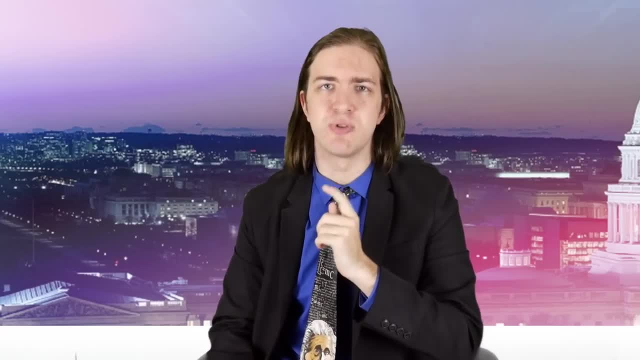 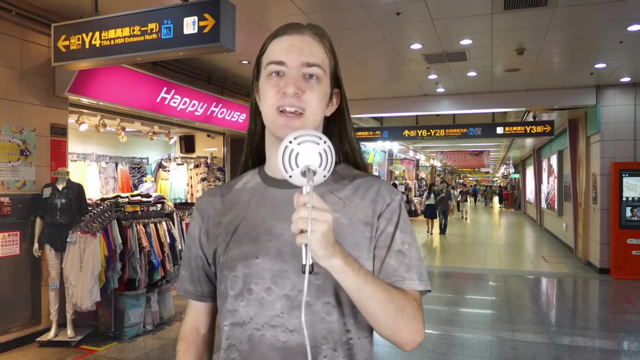 Windows has reported using Morning Brew to receive their daily news in a way that actually leaves them informed, fulfilled and hopefully not wanting to strangle someone Interesting. do tell us more about this Morning Brew thing. Morning Brew is a daily newsletter covering stories in business, finance and tech with witty.